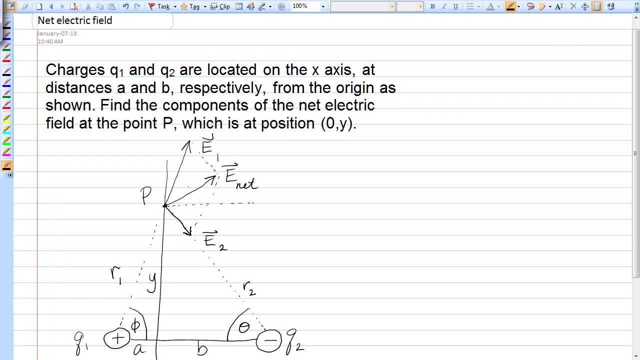 on my diagram. at my field point, E1 is an angle phi up from the x-axis and E2 is an angle theta down from the x-axis. Okay, now we'll find the magnitudes of E1 and E2 using the definition of the electric. 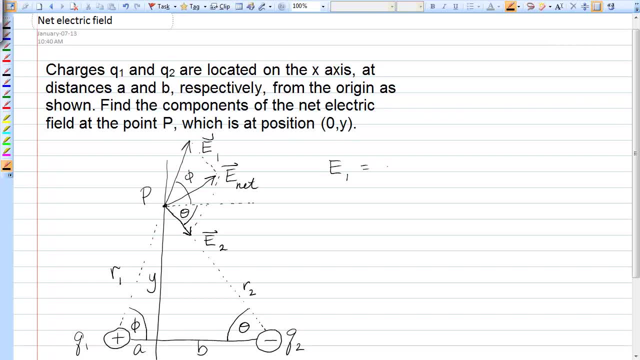 field due to a point charge. So the magnitude of E1 is equal to Coulomb's constant K times the magnitude of Q1 over the distance from the charge to the point of interest squared. And remember we can only use the letters that are given to us in the problem in. 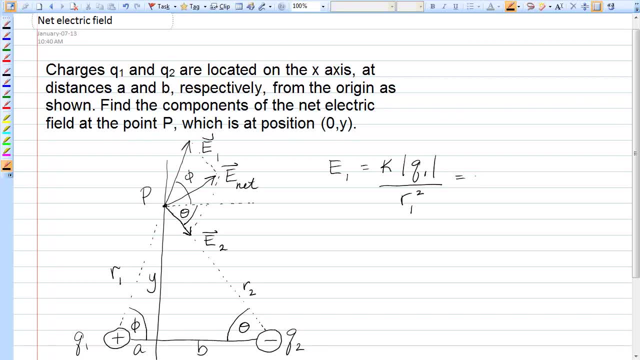 our answer. So we can use Q1, Q2, A, B and Y, but we can't use R1, theta or phi. So let's get R1 in terms of A and Y, and it would simply be A squared plus Y. 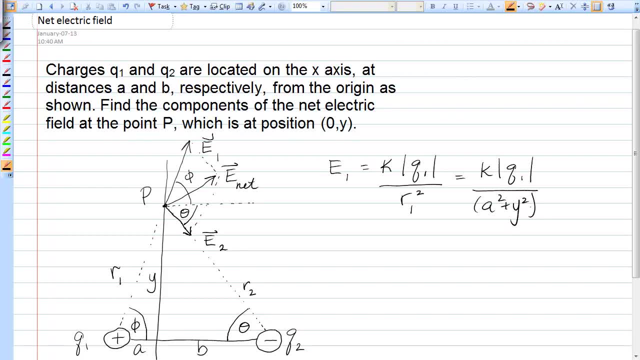 squared, square-rooted squared, so it's just to the 1 power Okay. similarly, E2, the magnitude is K magnitude of Q2 over R2 squared. so it's K magnitude of Q2, in this case it's B squared plus Y squared. 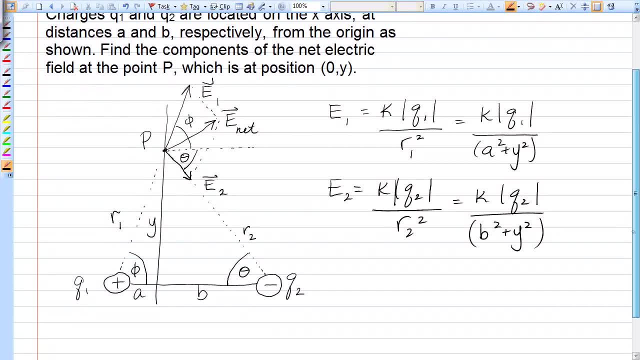 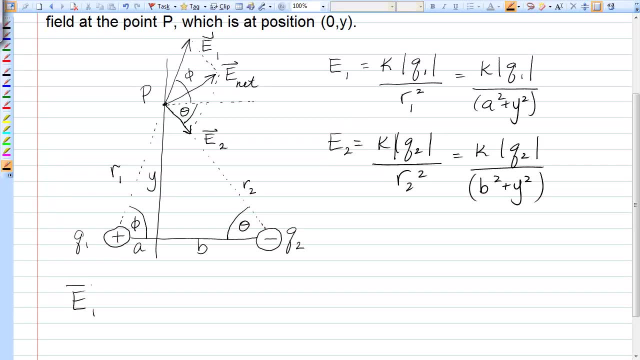 Now to get the components. I'm going to write these two electric field vectors in terms of their I hat, J hat components. So E1 vector will be the magnitude KQ1 over A squared plus Y squared times the cosine of phi for the X component, plus the magnitude times the sine of phi J hat, and similarly the. 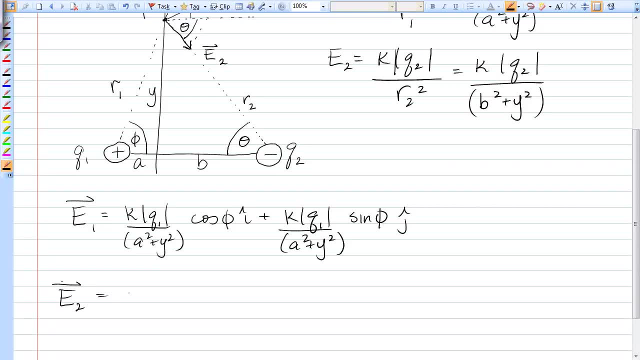 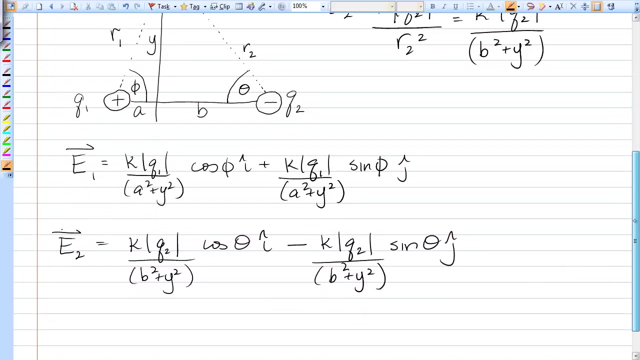 electric field due to Q2, is magnitude of that field times cosine of theta, this time, and then minus because the y component points down magnitude of b2 times the sine of phi theta. Okay now, as I said earlier, we cannot leave theta and phi in our answer. 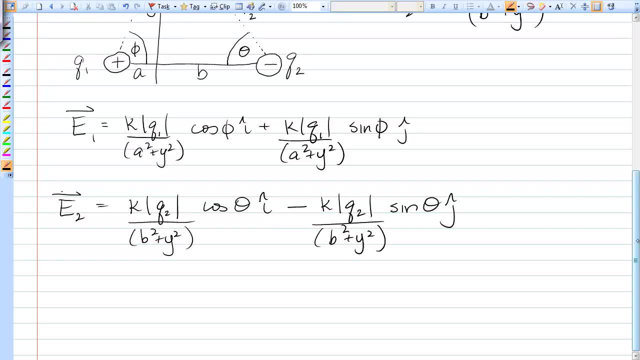 so let's get those in terms of the variables that we're given. So we can see from the triangle that the cosine of phi is equal to a over r1, which is a over the root of a squared plus y squared. Similarly, sine phi is equal to y over r1,. 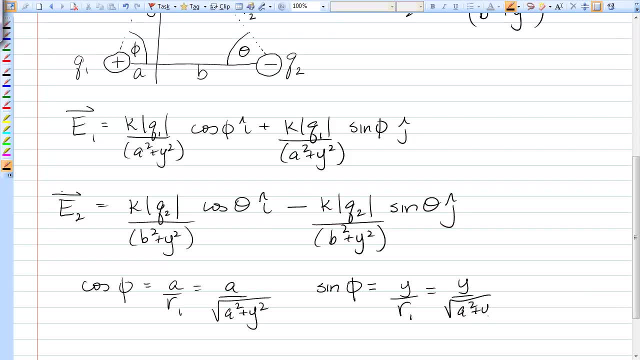 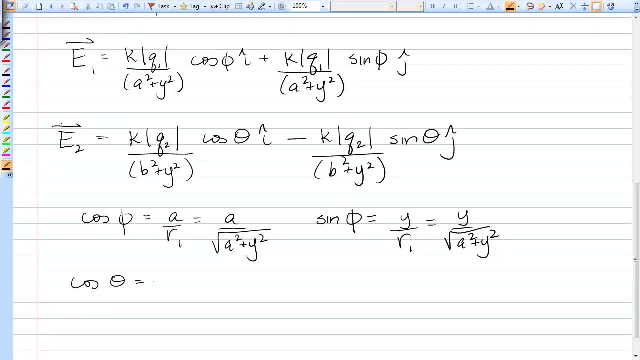 so it's y over the root. So it's y over the root of a squared plus y squared. And for theta we just substitute in b instead of a, so we have b over r2, so it's b over the root of b squared plus y squared. 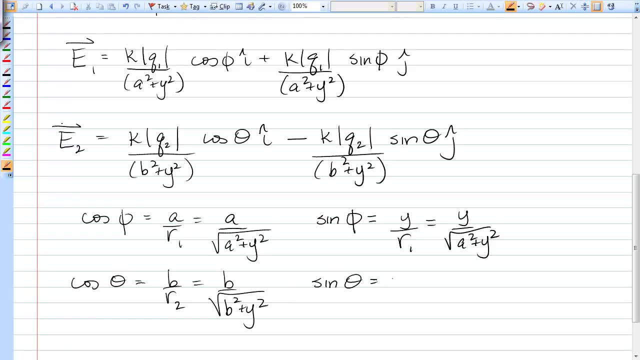 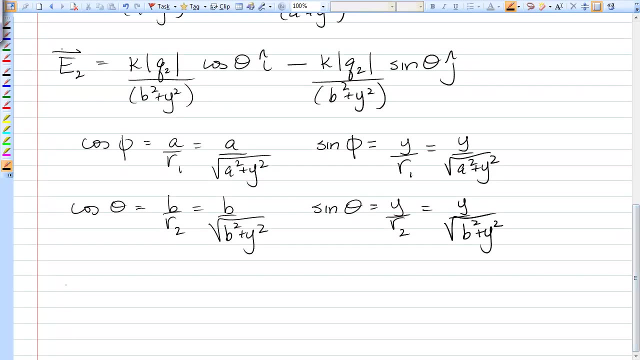 and sine theta is y over r2, so it's y over the root of b squared plus y squared. All right, let's substitute. We're going to add that into our components and I'll go right away to the net x component. 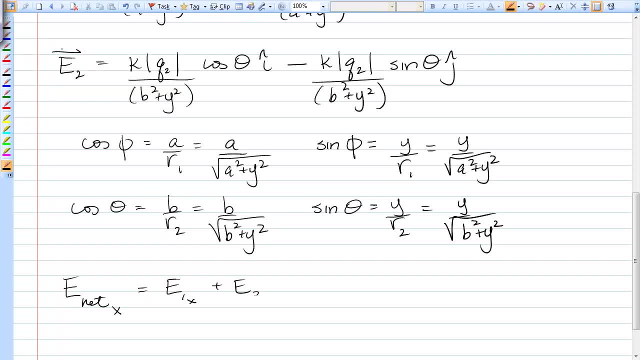 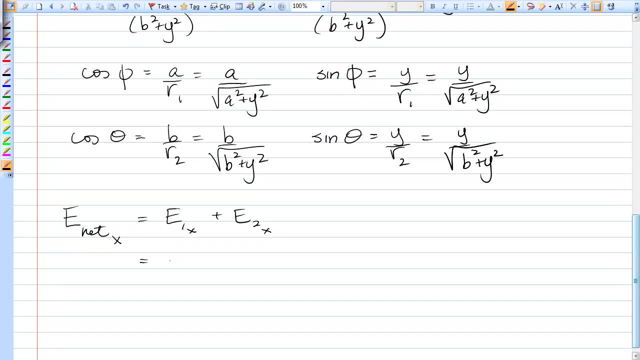 So it's the x component from 1 plus the x component from 2.. Okay, so the x component from 1 is k, magnitude q1, and then I'm going to substitute cosine phi in there And on the bottom. now I'm going to have 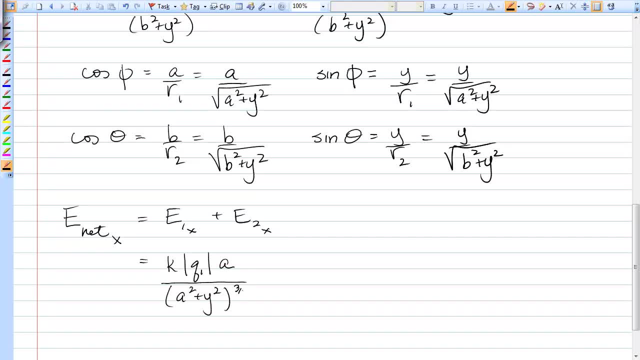 I'm going to have a squared plus y squared to the 3 halves, because 1 plus 1 half is 3 halves. And then for the second electric field, I've got q2, b, and now it's b squared plus y squared to the 3 halves. 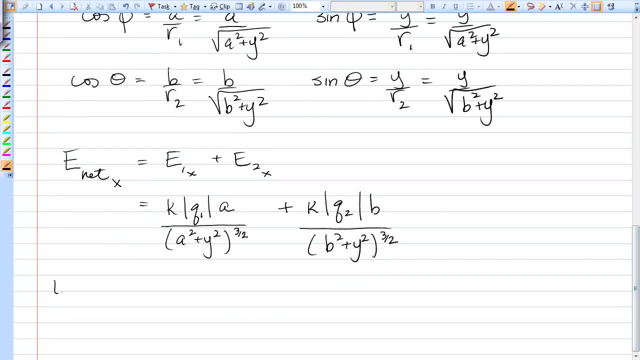 Okay, that's the x component and then the y component. doesn't look too different. That's magnitude, The first one. now I've got a y instead of an a, but I still have the 3 halves on the bottom and I have a minus here. 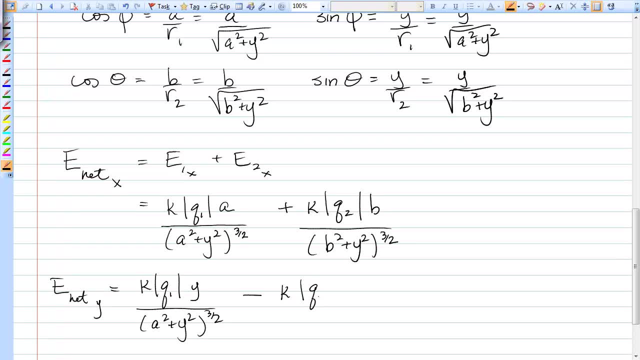 plus the y component of b, two points down squared plus y, squared to the 3 halves, And that's our final answer.